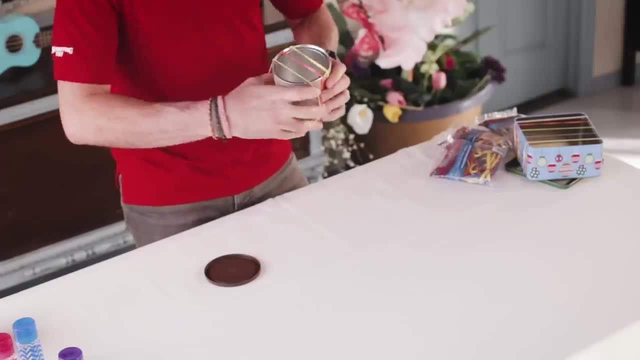 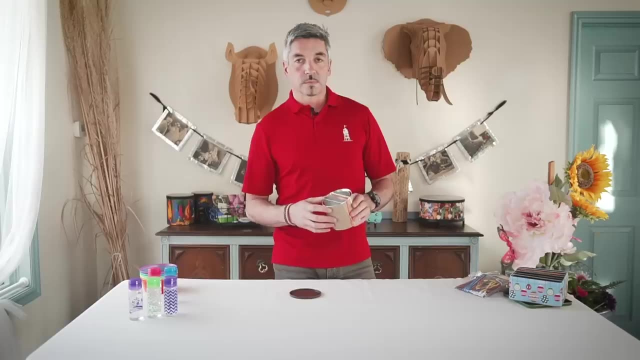 with more rubber bands. So depending on the thickness and how tight they are, they're going to sound different. So remember the pitch depends on the thickness of the rubber band, but also how tight it is. If it's in the middle it's going to be tighter than the ones on the 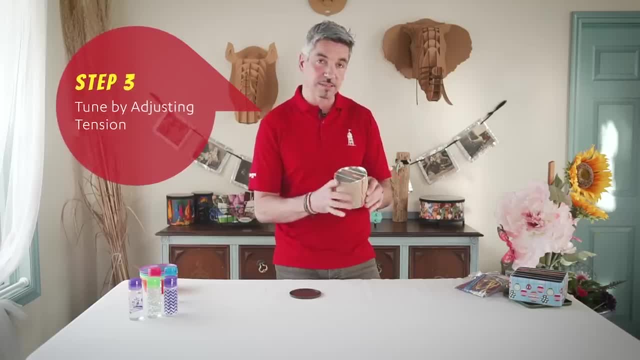 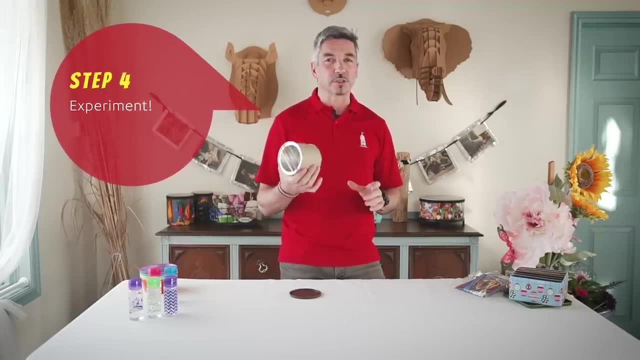 side. but you can tune it by pulling them. you can possibly tape them down and that's going to change the sound that it makes. So remember, this is all about experimenting, trying different containers. try different size rubber bands, different tensions. see how many different sounds you can create. We can. 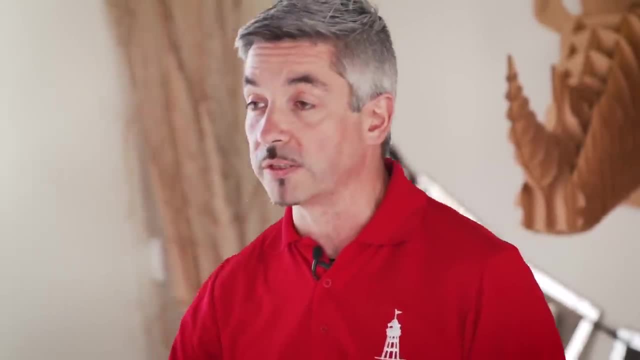 also make a very simple wind instrument, also using common household items. So a wind instrument is a square piece of wood. you can carefully cut it into small pieces and then common household items. So wind instrument is any instrument where the vibration is causing by air. 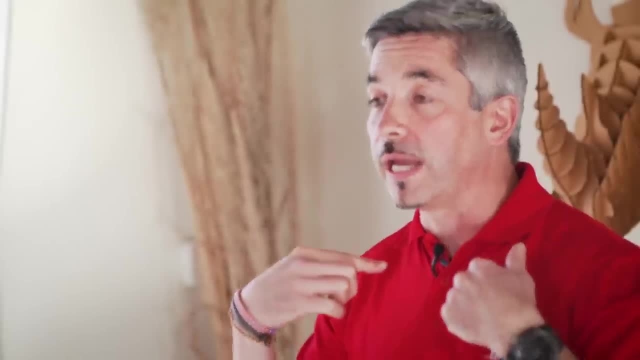 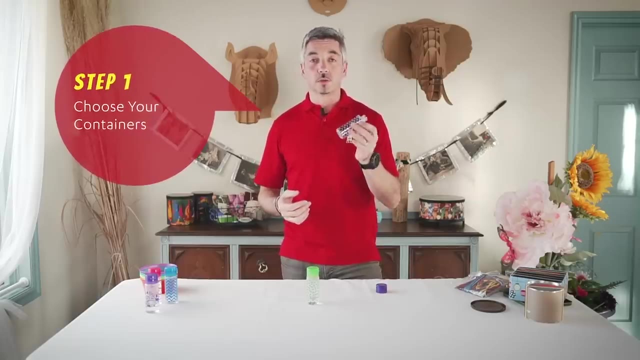 moving through it. So just like our voice creates sound by air traveling across our vocal cords, we can create sound with other things, like this shampoo bottle. So it's not going to vibrate quite the same way. What happens is that if we blow across the top, it's going to split the air with 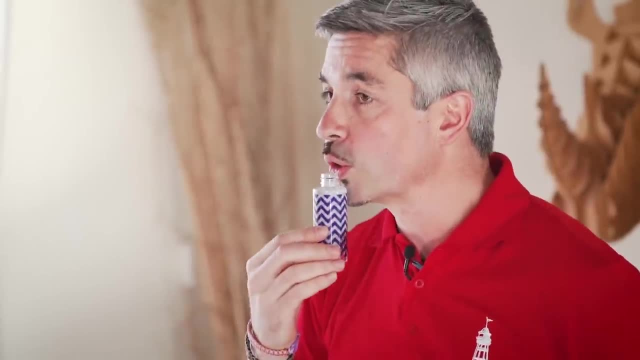 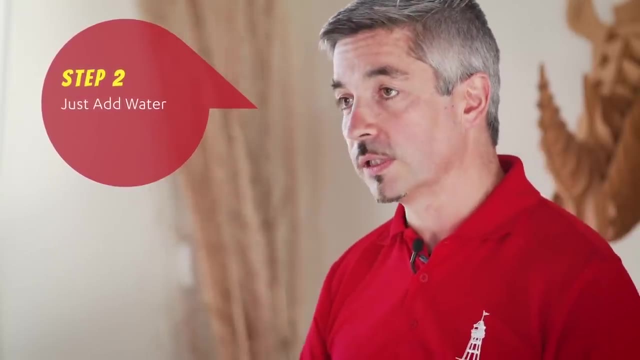 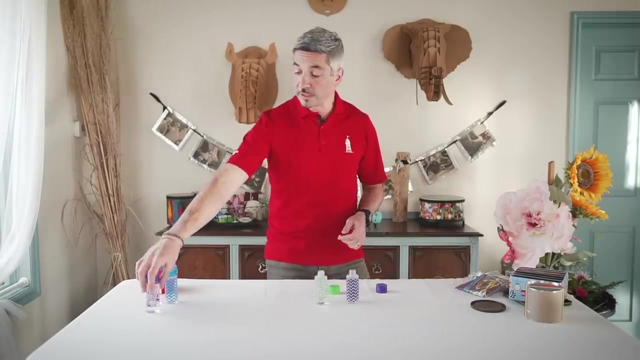 some of the air going across and some of the air going inside. it Like so: Now, if we fill this bottle with different levels of water, we're going to create a different sound, because the air inside doesn't have to travel as far. So we can use this to create an instrument by 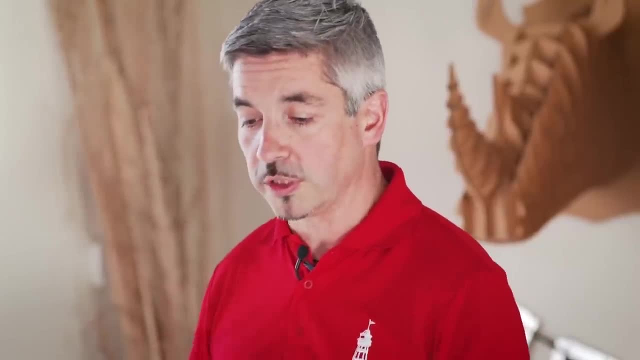 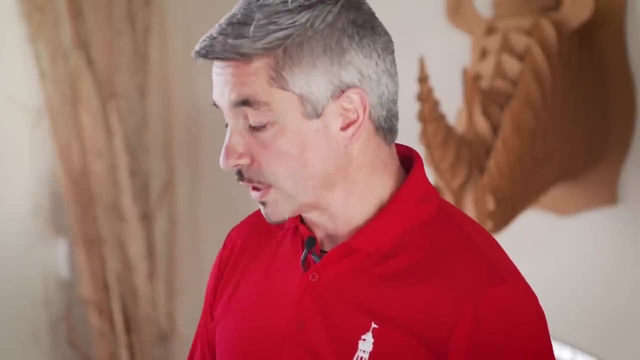 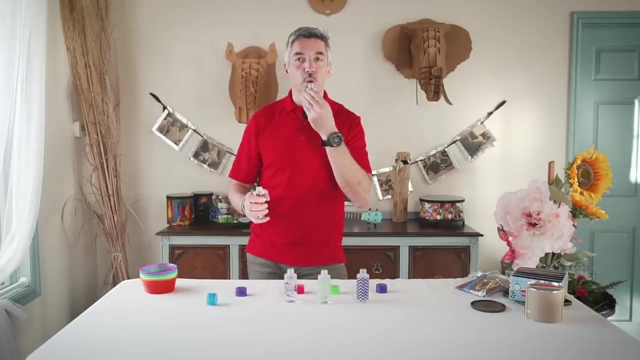 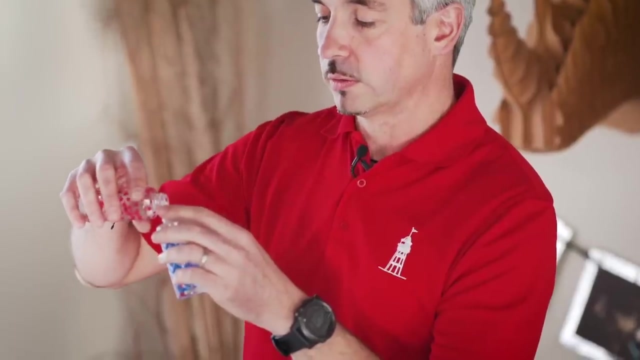 using different amounts of water in different bottles. So here we have three notes. So by adjusting the water level in those bottles we're going to to create different pitches and different notes. So if we start with an empty bottle, remember, and we fill it with water a little bit and fill it more. 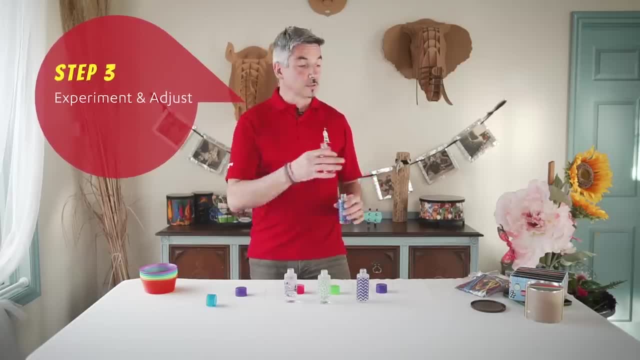 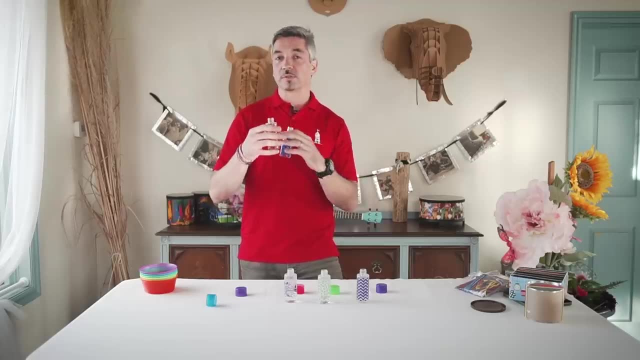 So remember this is all about experimentation. You know the principles to create your own string or your own wind instrument. Now you can experiment with different containers, different rubber bands, different levels of water and make different pitches. So if you enjoyed this video, don't forget to like. 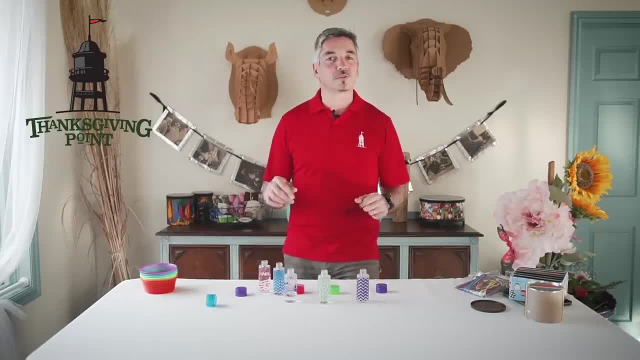 it. You can subscribe to our channel. If you make some great instruments or if you have any questions, you can leave them in the comments and, of course, don't forget to share with your friends.